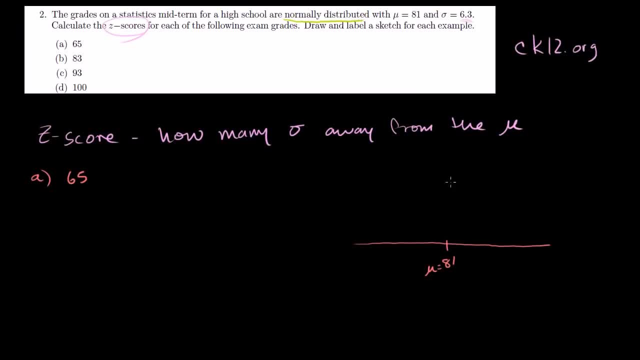 So our distribution? They're telling us that it's normally distributed, So I can draw a nice bell curve here. They're saying that it's normally distributed, So that's as good of a bell curve as I'm capable of drawing. This is the mean right there at 81.. 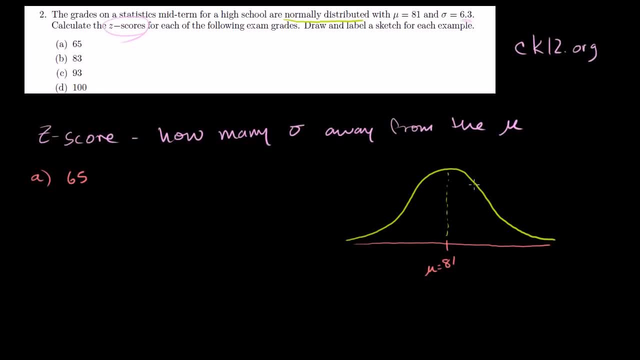 And the standard deviation is 6.3. So one standard deviation above and below is going to be 6.3, away from that mean. So if we go 6.3 in the positive direction, that value right there is going to be. 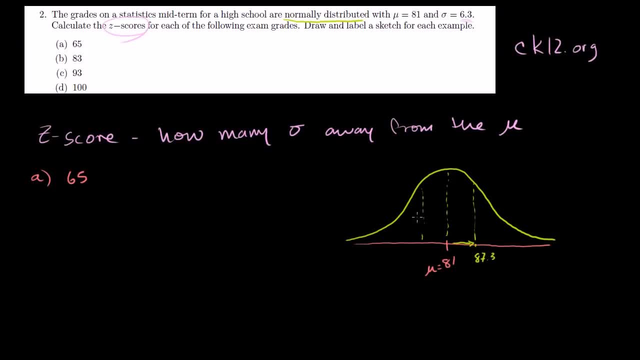 It's going to be 87.3.. If we go 6.3 in the negative direction, where does that get us? That goes to what? 74.7.. If we add 6, it'll get us to 80.7.. 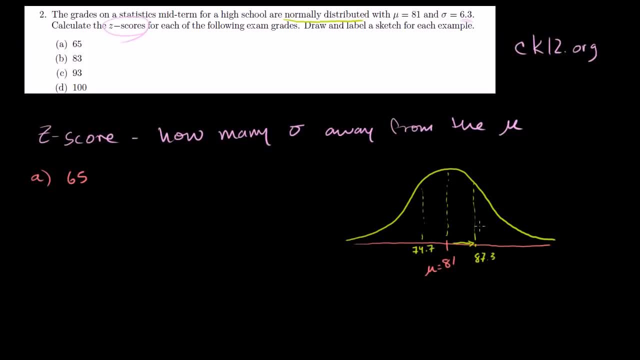 And then 0.3 will get us to 81. So that's one standard deviation below and above the mean, and then you would add another 6.3 to go to two standard deviations, so on and so forth. So that's at least a drawing of the distribution itself. 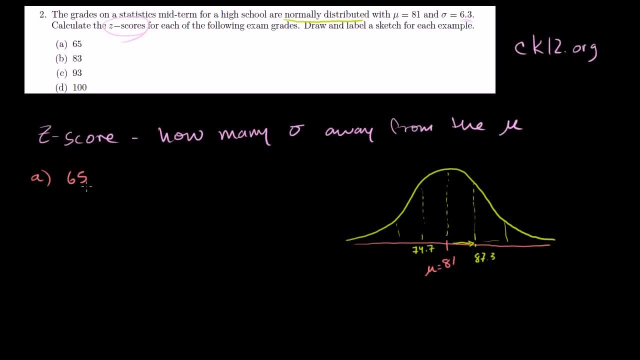 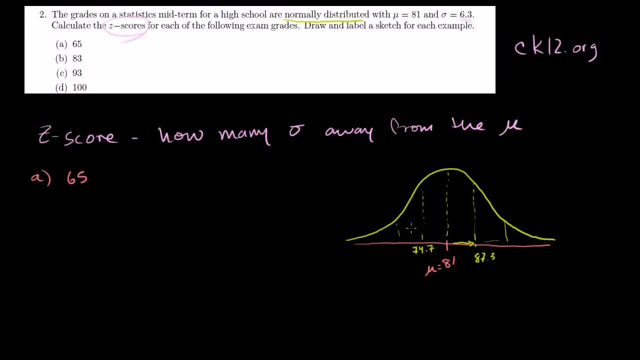 So 65 for each of these grades. 65 is how far 65 is, you know, it's maybe going to be here someplace. So we first want to say: well, how far is it? just from our mean, from our mean. 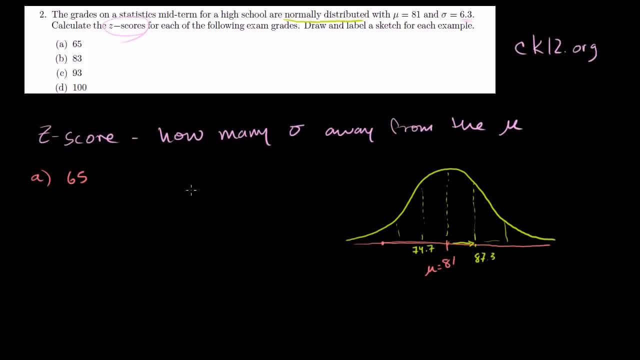 So the distance is? we just want a positive number here. Well, actually you want a negative number because you want your z-score to be positive or negative. Negative would mean to the left of the mean and positive would mean to the right of the mean. 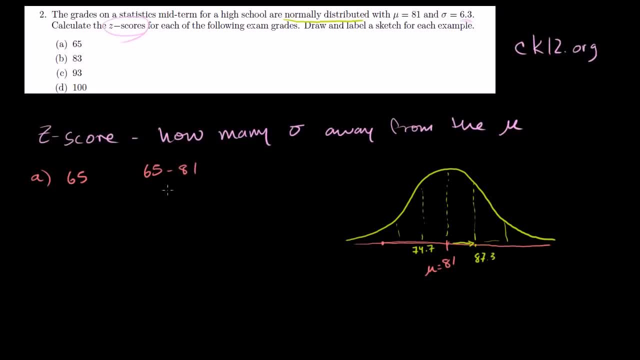 So we say 65.. Minus 81.. So that's literally how far away we are. but we want that in terms of standard deviations, So we divide that by the length or the magnitude of our standard deviation. So 65 minus 81.. 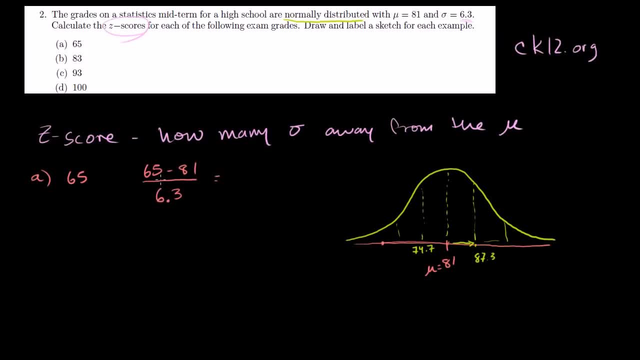 Let's see: 81 minus 65 is what It is, 5 plus 11. It's 16.. So this is going to be minus 16 over 6.3, and take our calculator And let's see if we have minus 16 divided by 6.3,. you. 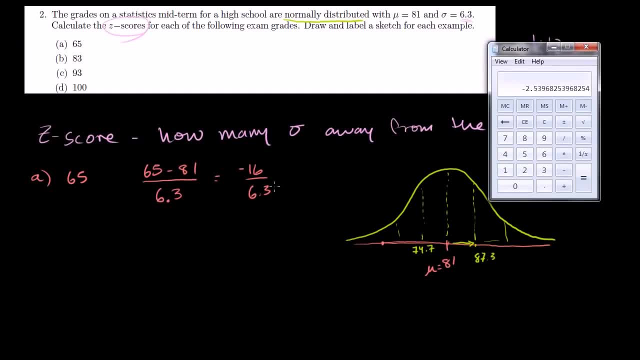 get minus 2.54.. So approximately equal to minus 2.54.. That's the z-score for a grade of 65.. Pretty straightforward. Let's do a couple more. Let's do all of them- 83.. So how far is it away from the mean? 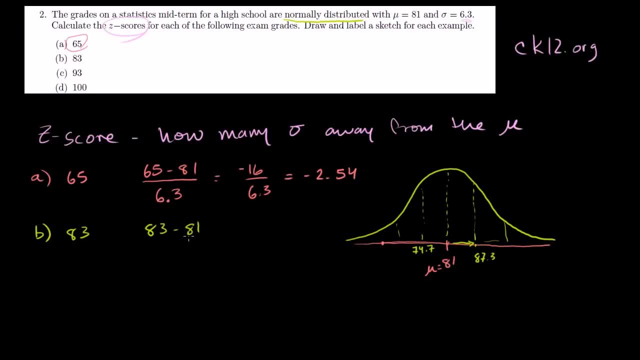 Well, it's 83.. Minus 81. It's 2 grades above the mean, But we want it in terms of standard deviations. How many standard deviations? So this was part a. a was right here. We were at 2.5 standard deviations below the mean. 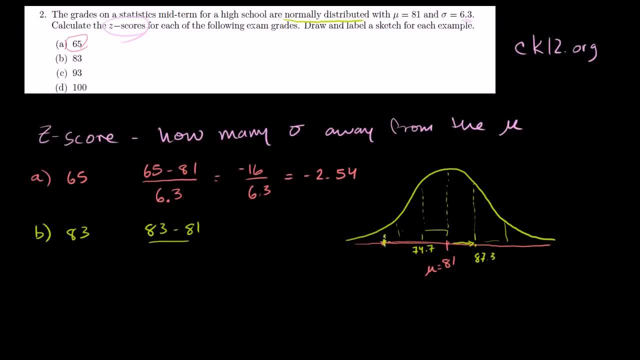 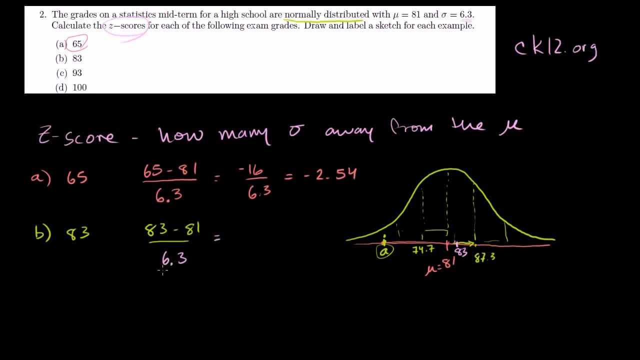 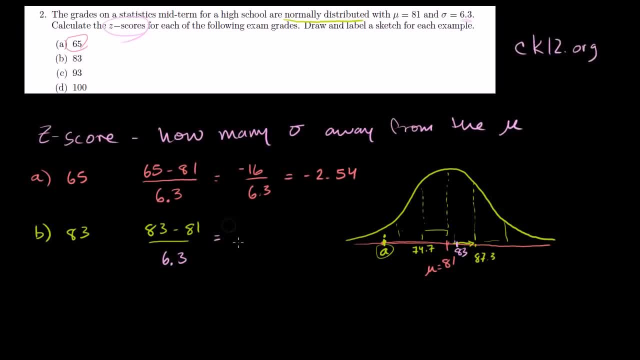 0.32 roughly, So here we get 0.32.. So 83 is 0.32 standard deviations above the mean. So it would be roughly 1 third of the standard deviation along the way. right, Because this was one whole standard deviation. 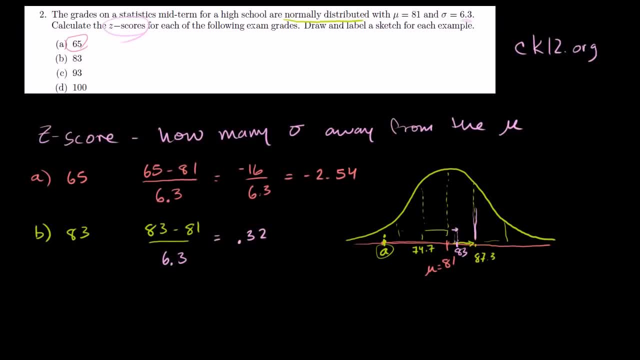 So we're 0.3 of a standard deviation above the mean. Choice number C Or not. choice part C. I guess I should call it 93.. Well, we do the same exercise. 93 is how much above the mean? 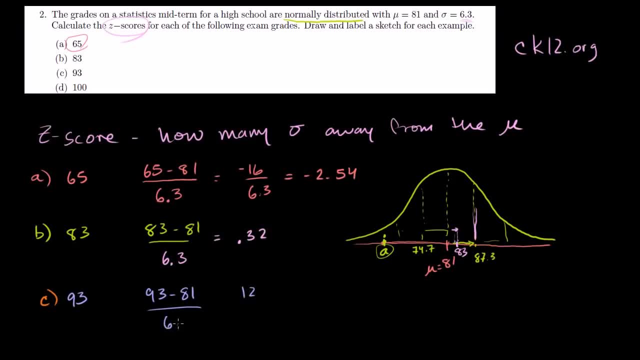 Well, 93 minus 81 is 12.. But we want it in terms of standard deviation. So 12 is how many standard deviations above the mean? Well, it's going to be almost 2.. Let's take the calculator out. 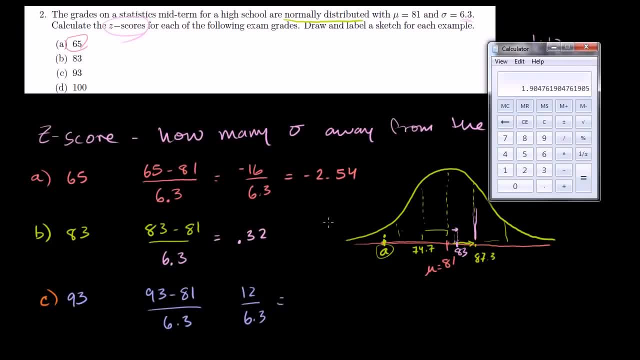 So if we get 12 divided by 6.3, it's 1.9 standard deviations. Its z-score is 1.9, which means it's 1.9 standard deviations above the mean. So the mean is 81.. 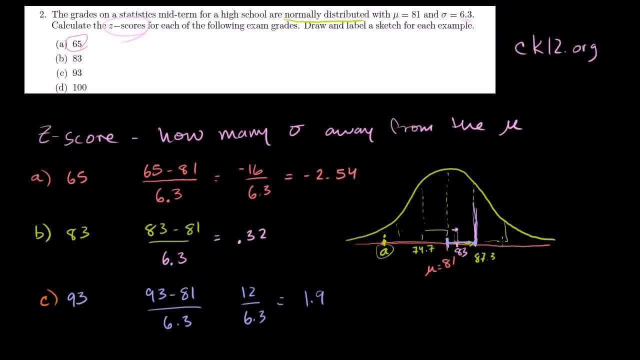 We go one whole standard deviation and then 0.9 standard deviations, And that's where a score of 93 would lie. right there Its z-score is 1.9.. All that means is 1.9 standard deviations above the mean. 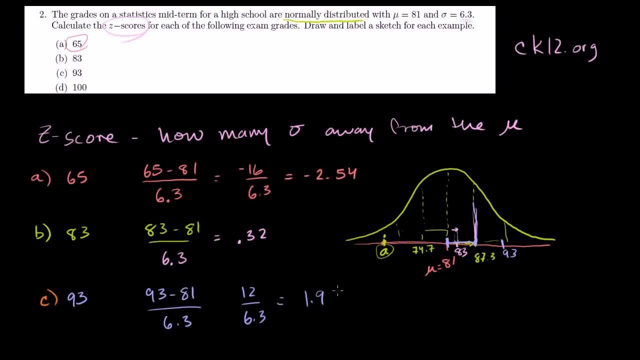 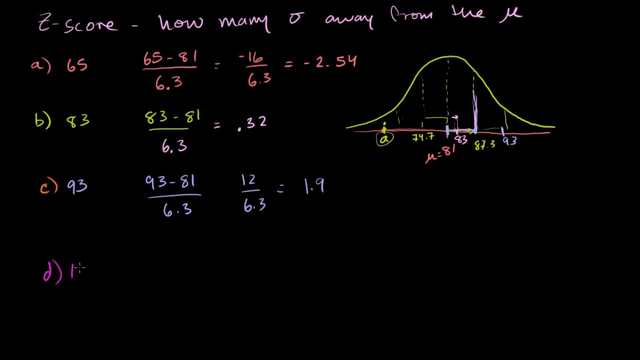 Let's do the last one. I'll do it in magenta D, part D: Score of 100.. We don't even need the problem anymore. A score of 100. Well, same thing, We figure out how far is 100 above the mean. 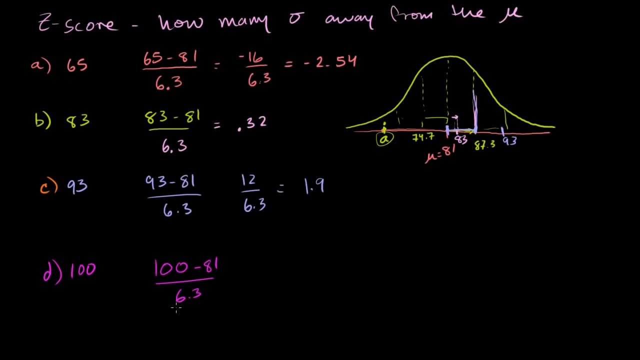 Remember the mean was 81. And we divide that by the length or the size or the magnitude of our standard deviation. So 100 minus 81 is equal to 19 over 6.3. So it's going to be a little over 3 standard deviations. 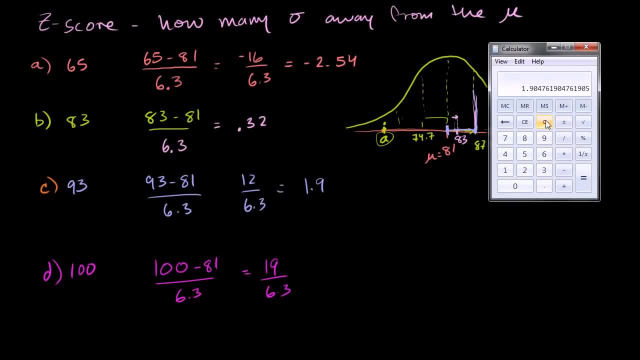 In the next problem we'll see. what does that imply in terms of the probability of that actually occurring. But if we just want to figure out, the z-score, 19 divided by 6.3 is equal to 3.01.. So it's very close. 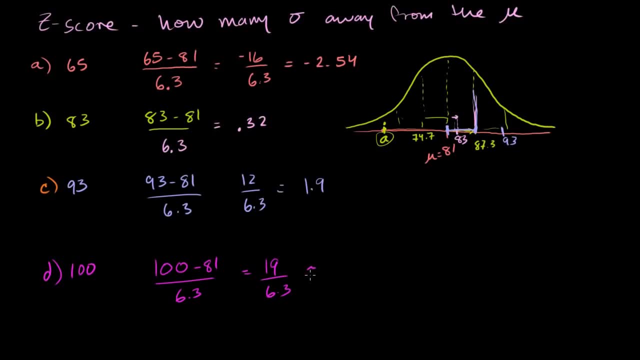 3.02, really, if I were to round So it's very close to 3.02.. Its z-score is 3.02, or a grade of 100 is 3.02 standard deviations above the mean. So remember this was the mean, right here. 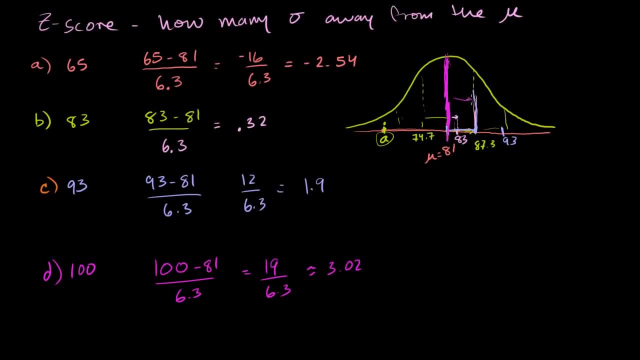 Right here at 81.. We go one standard deviation above the mean, two standard deviations above the mean. The third standard deviation above the mean is right there. So we're sitting right there on our chart a little bit above that: 3.02 standard deviations above the mean. 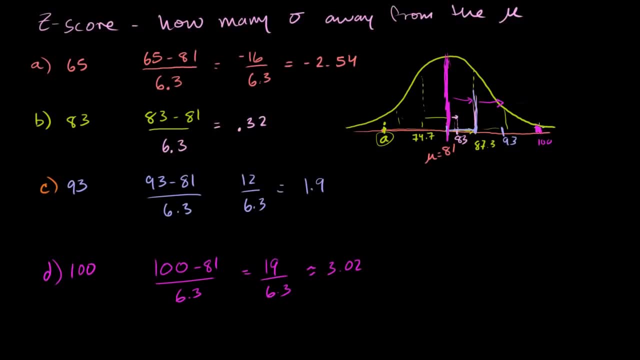 That's where a score of 100 would be And you can see the probability, the height of this. that's what the chart tells us. It's actually a very low probability, And actually not just a very low probability- of getting something higher than that, because we've learned before. 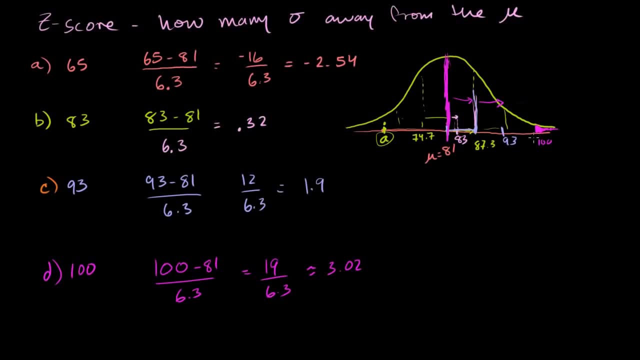 in a probability density function, the probability if this is a continuous, not a discrete, the probability of getting exactly that is 0.. If this wasn't discrete, But since this is a score, as in a test, we know that it's. 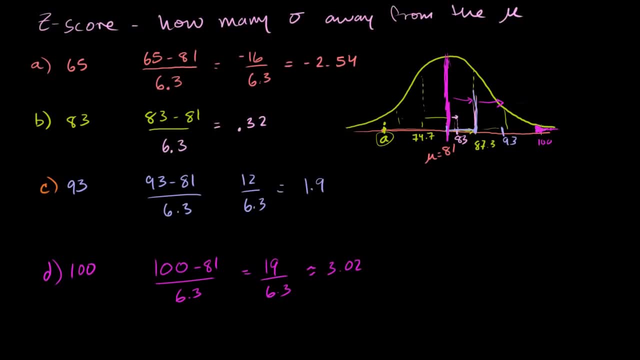 actually a discrete probability function, But the probability is low of getting higher than that, because you can see where we sit in the bell curve. Well anyway, hopefully this at least clarified how to solve for z-scores, which is pretty straightforward mathematically. 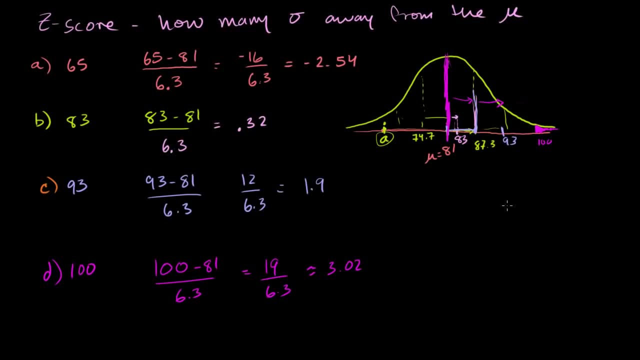 And in the next video we'll interpret z-scores and probabilities a little bit more.